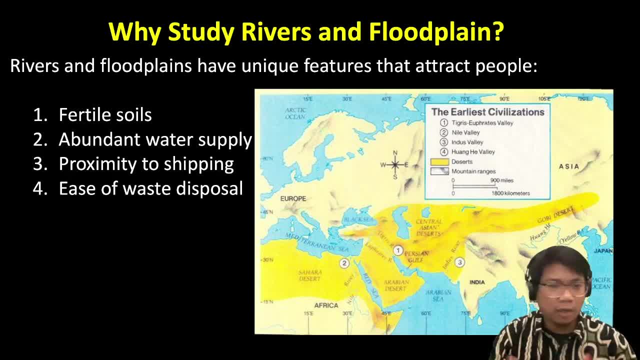 why humans like to be in the proximity of rivers. the reason is very simple: because the river can provide us with many things. It can provide us with fertile soils, so it's very good. The soils would be very good for agricultures. Of course, we know that it will supply lots of water, and proximity to shipping is also an important factor here, because obviously it will be a lot easier to transport goods from one point to the next. 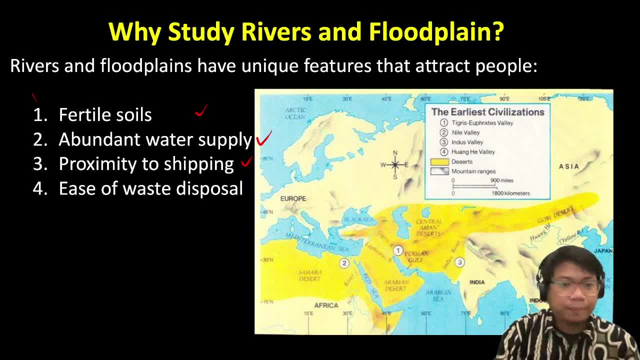 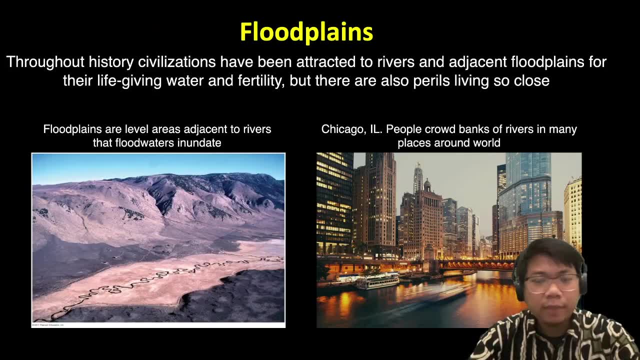 Maybe another city down the stream, for example, And it's also good for ease of waste disposal- Another reason for why humans like to live near a river, or why humans like to occupy flat plains. one of the main reasons for that is because flat plains are level areas, So it's very flat in terms of the shape of the river. 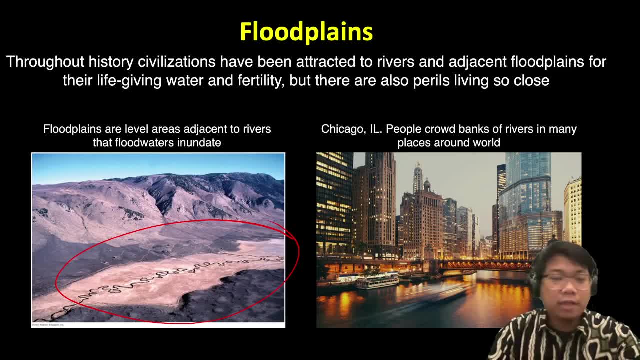 So, as you can see here on the left side here it actually shows flat plains of a major river. So we have a river right here in the middle that flows with lots of supply of water right here And look at the land adjacent to it. These are all flat plains And look how flat they are. So it's a lot easier for humans to build things right on that flat areas And that is the reason why humans like to live near flat plains. 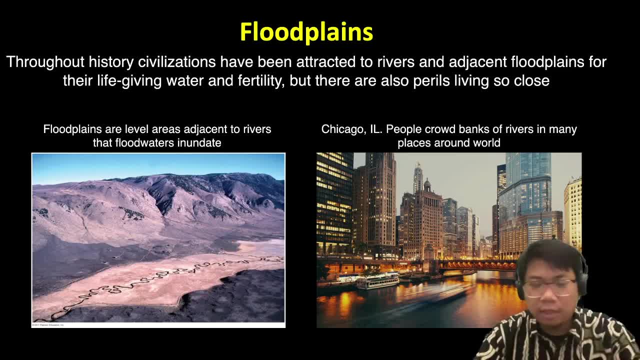 And that is the reason why humans like to live near flat plains. We also have a major river that flows right by the city, which is called the Raritan River, So there's a lot of human development population that actually occupies the land adjacent to rivers for many reasons that I've already mentioned. 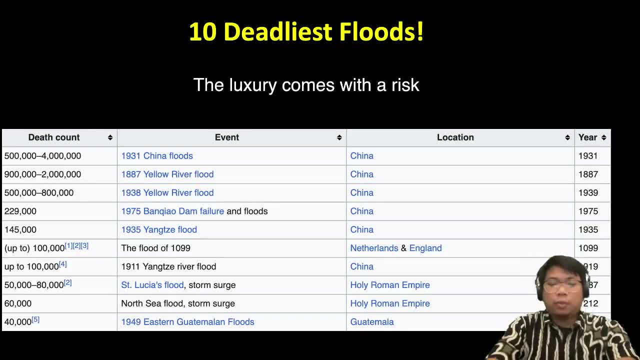 However, living next to the source of water, Water can come with a major risk, And here's the list of 10 deadliest floods that have occurred in human history. And the deadliest one happened in China in 1931, right here. that claimed almost up to 4 million people in one event. 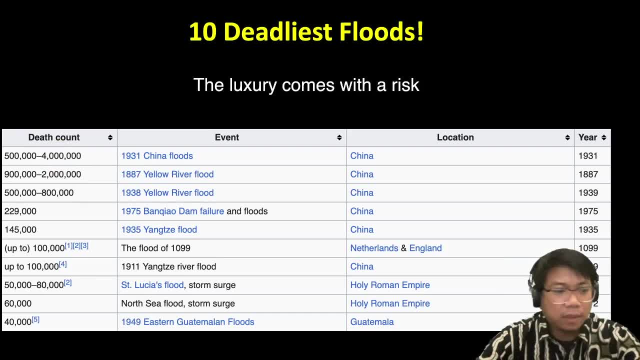